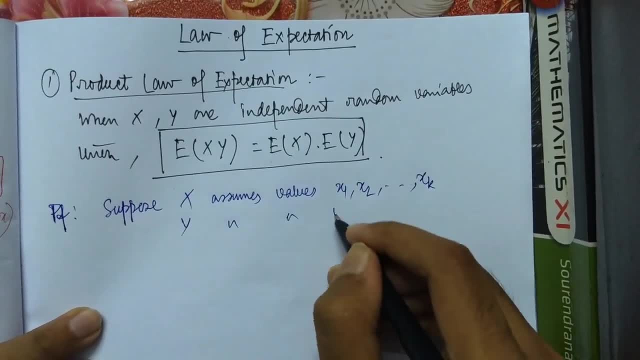 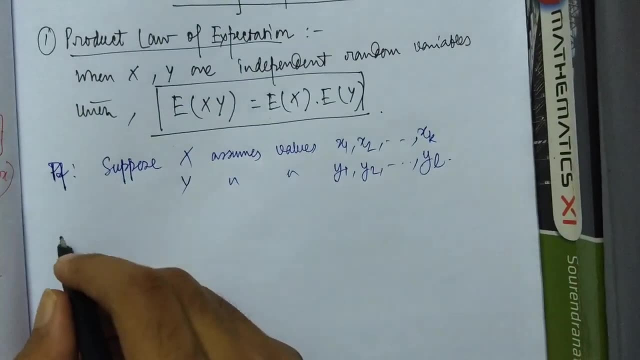 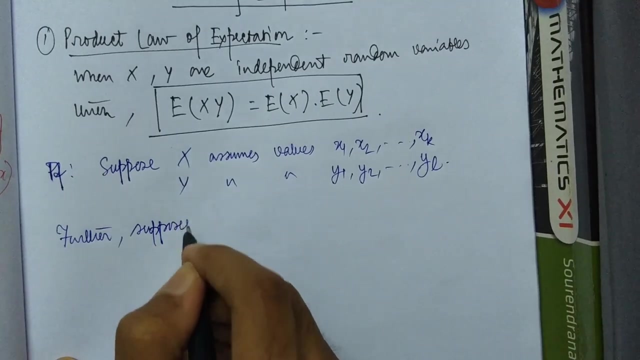 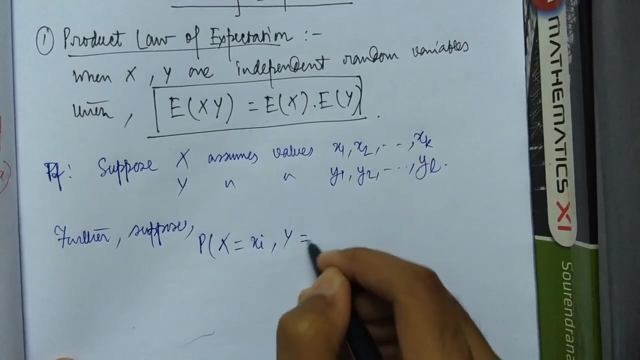 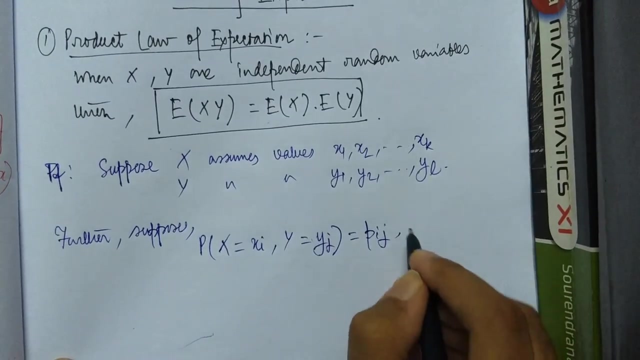 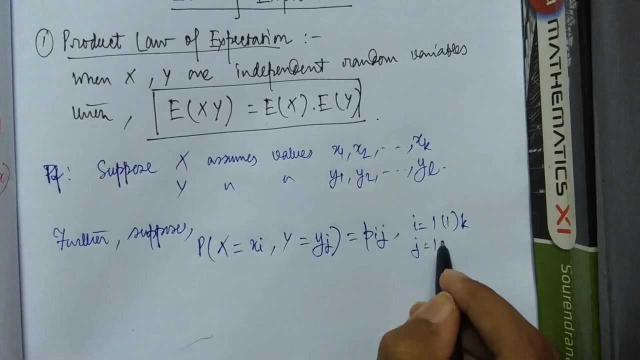 xk and y assumes values y1, y2 like this, up to yl Again. let us say further. suppose p of x equals to xi comma, y equals to yj, equals to pij, Where i runs from 1 to k. that means i equals to 1 to up to k and j runs from 1 to l, 1 to up to l. 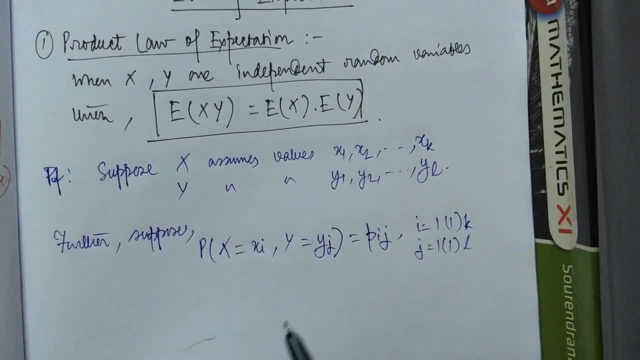 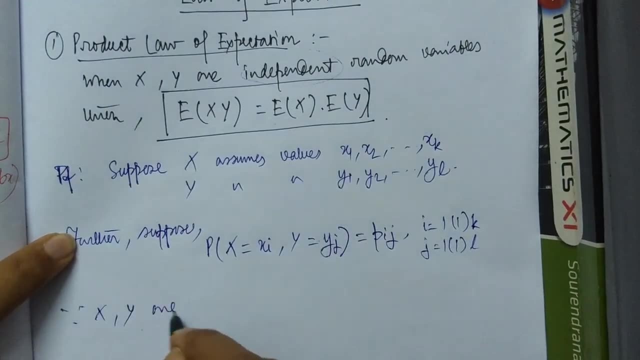 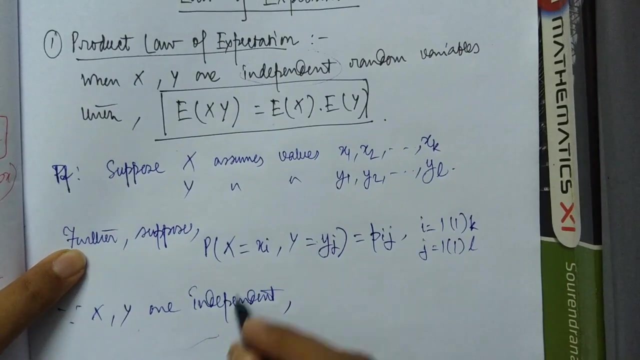 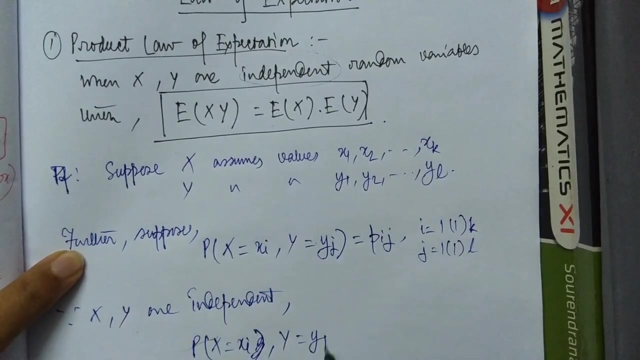 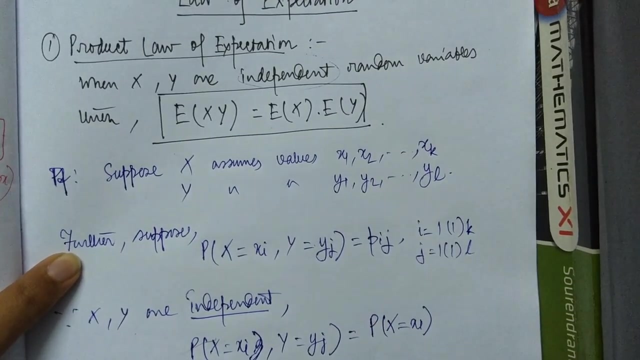 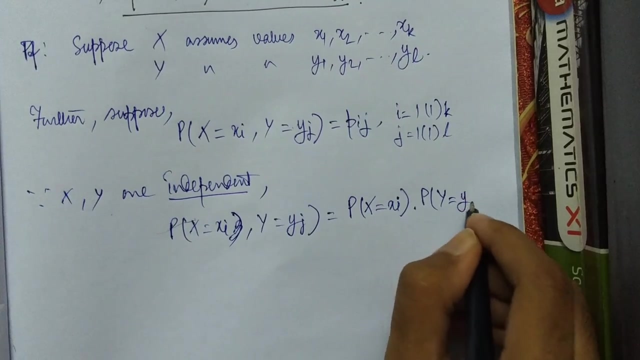 This is our consideration. Now it is said that x and y are independent. Since x comma y are independent, we have this expression: X- I- sorry- comma Y equals to Y, J. since they are independent, these can be written separately, which means P- X equals to X, I into Y, equals to Y, J. 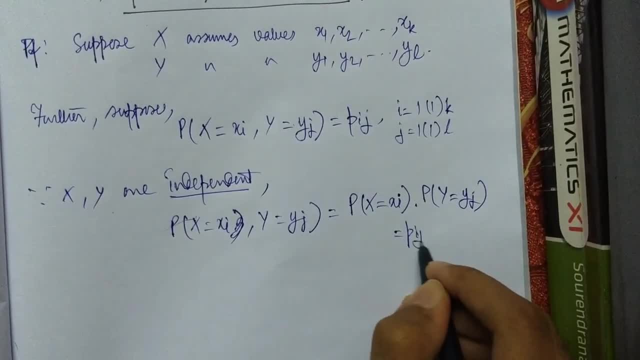 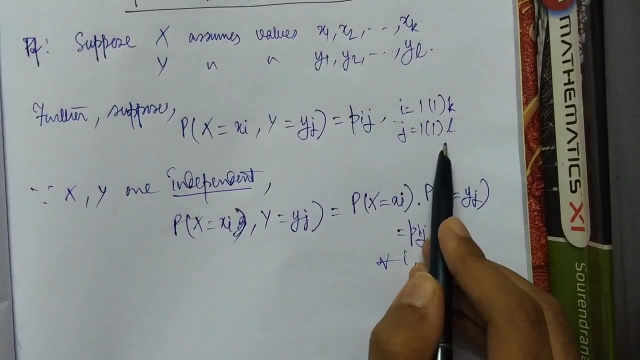 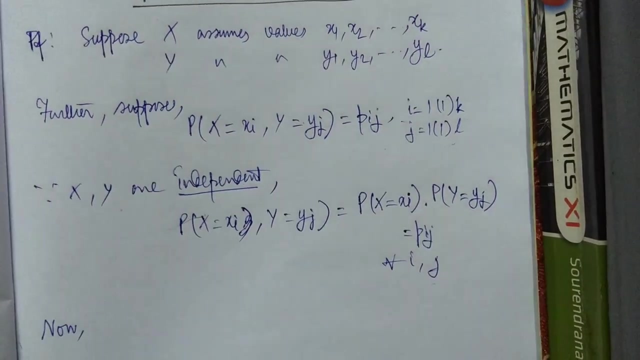 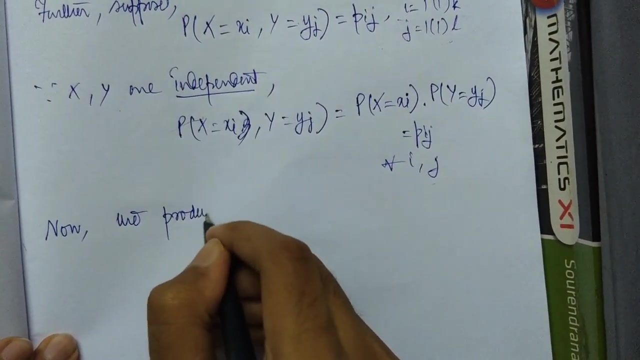 this equals P, I, J, done for all I comma J, which runs from 1 to K and 1 to L. now, now we have in here the product XY, since this is a product log, so obviously we would require to find the product. the product XY is also a random variable. 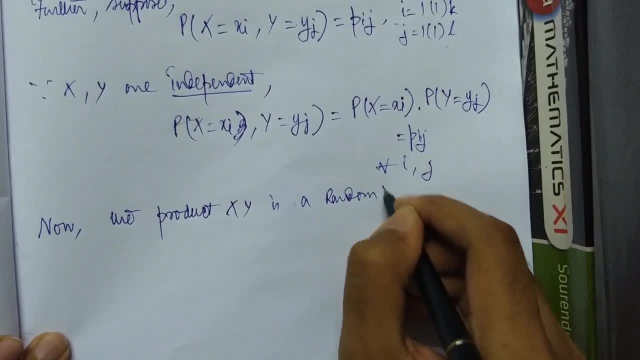 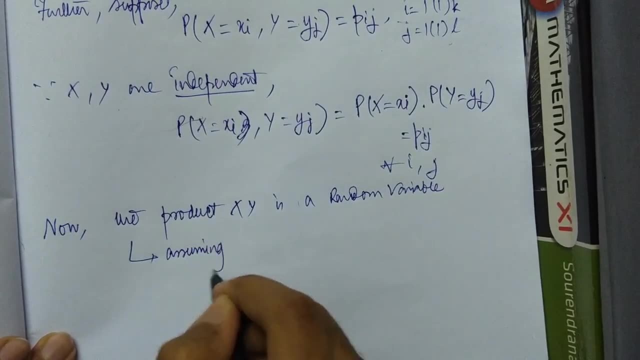 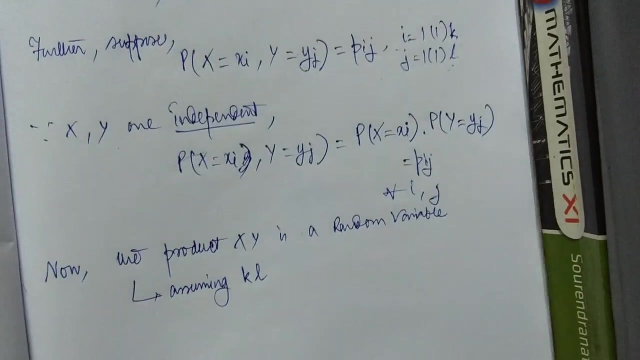 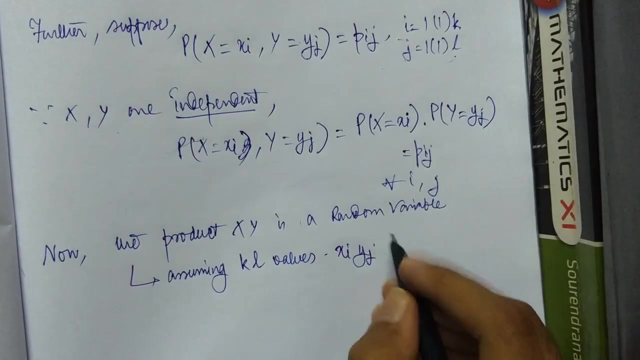 here we are going to write product X in the product space. so the product X in the product space is a random variable variable and they assume assuming k l values, since i runs from 1 to k and j runs from 1 to l, so in total they assume k l values, x, i, y, j having respective probabilities. 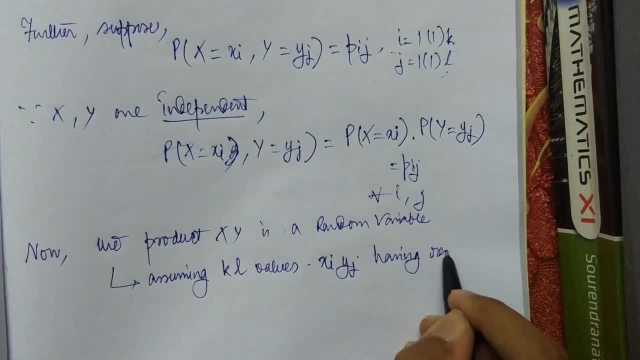 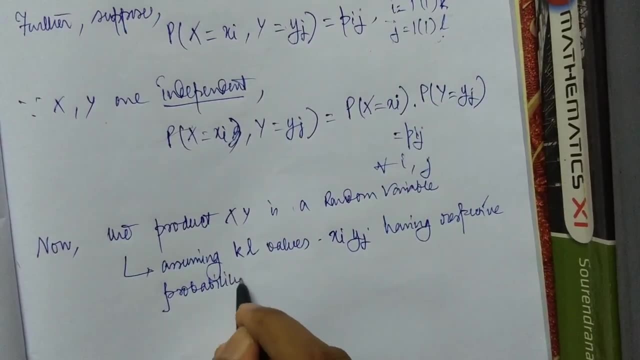 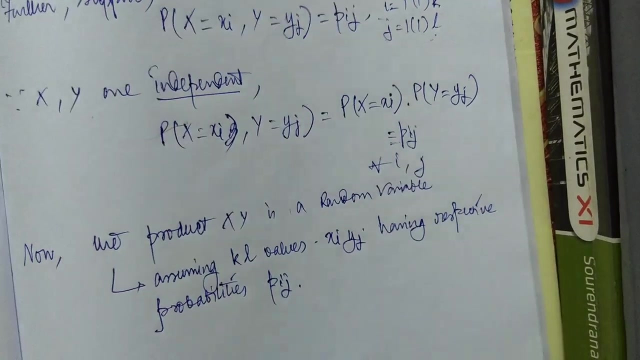 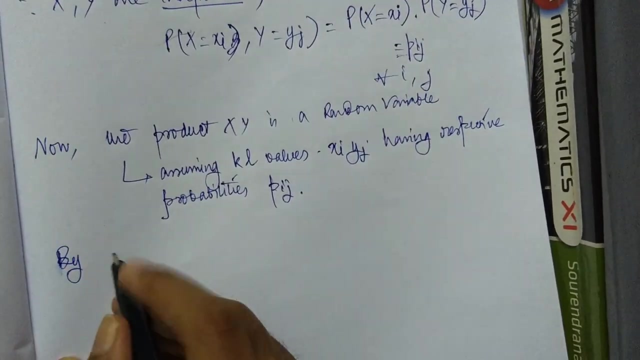 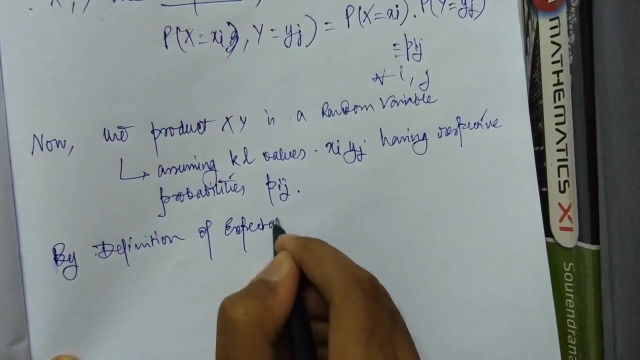 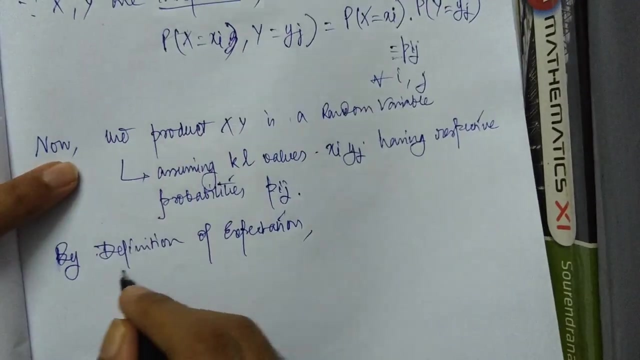 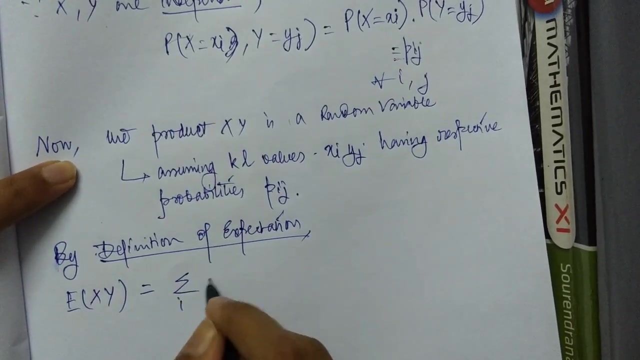 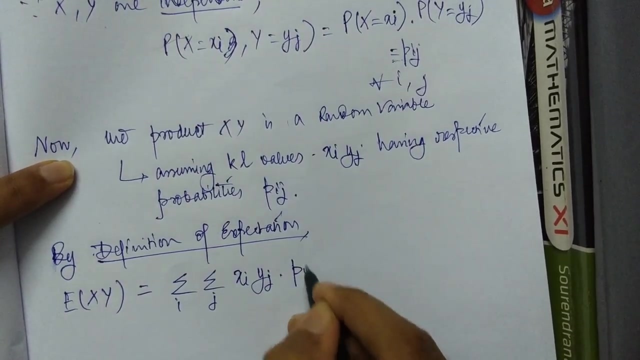 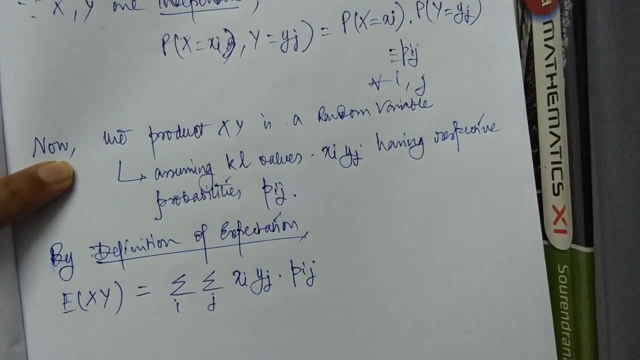 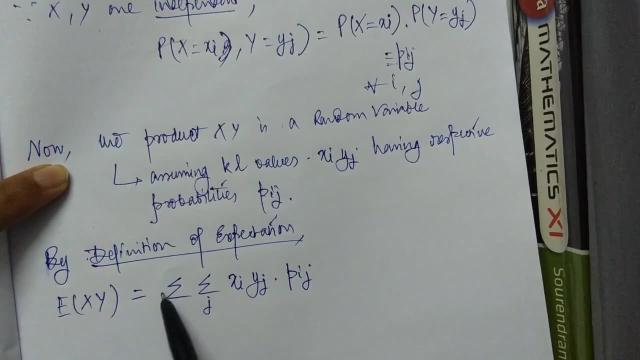 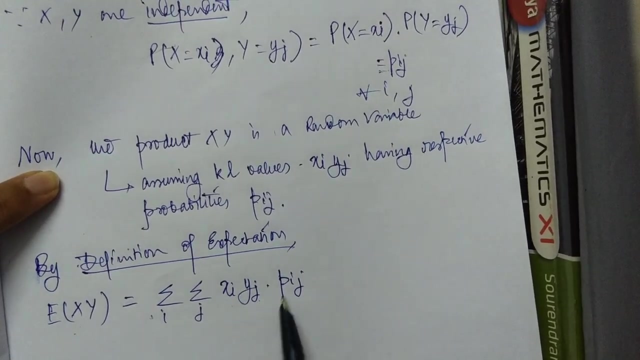 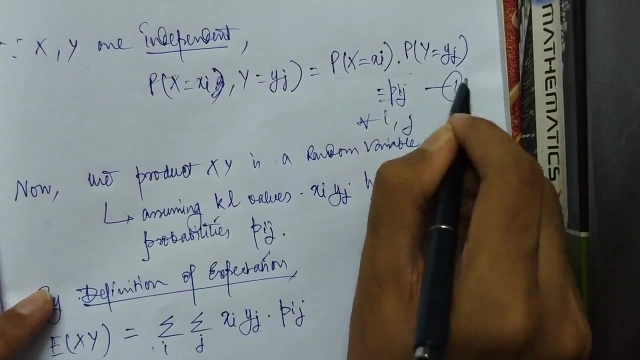 so, so, so, so so. summation, or the integration of all possible set of values of random variable. so since here we are taking summation, so the by the definition here goes that the expectation is equals to the summation of x, i, y, j into p i j. now we have gotten from here that let us suppose name this as one. 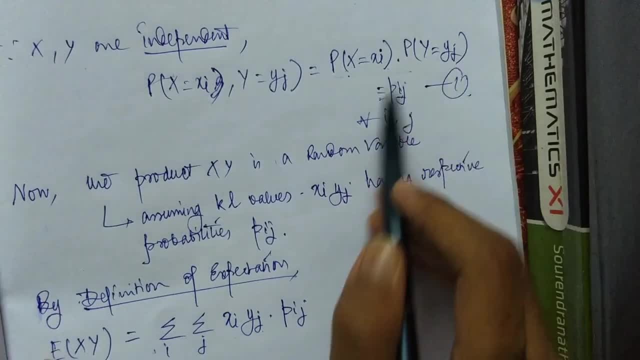 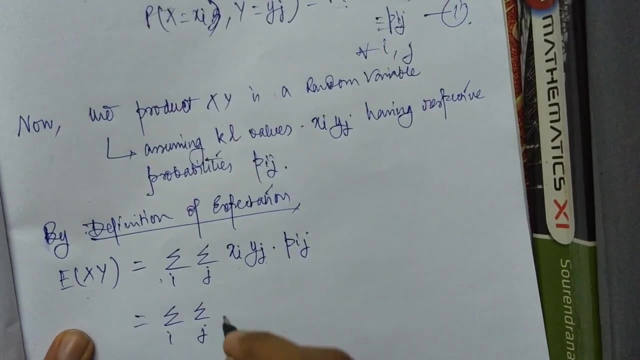 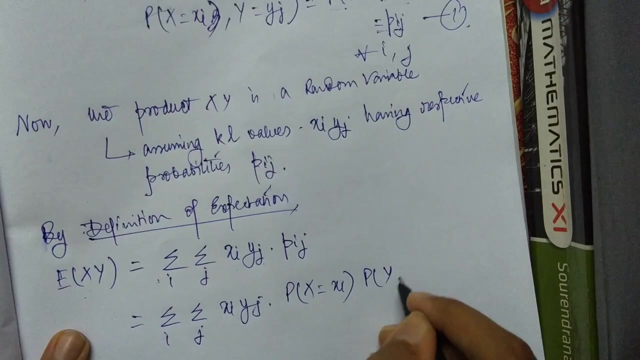 that p i j equals to p x, into x i, into p y, into y i, and so we will put this in here. what we have: i j, x, i y j. p i j is replaced by p x equals to x i and p y equals to. 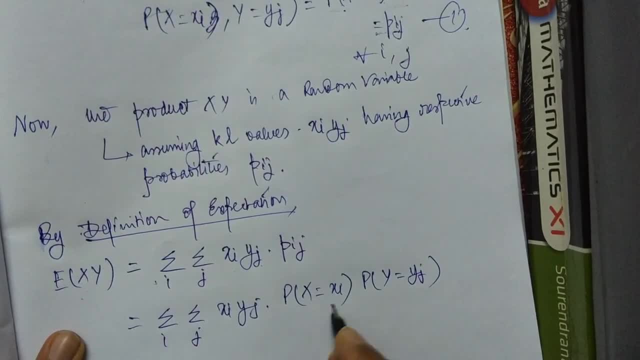 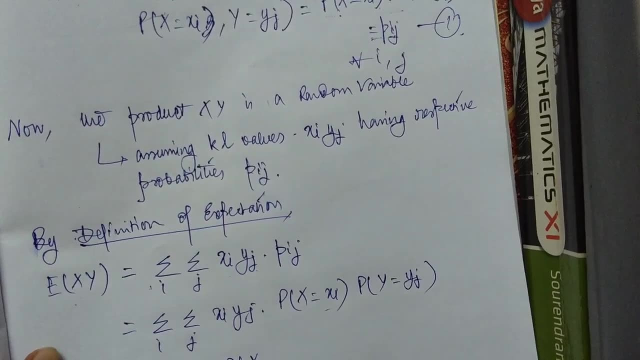 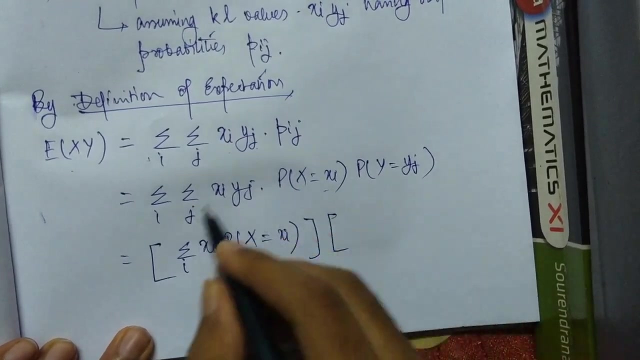 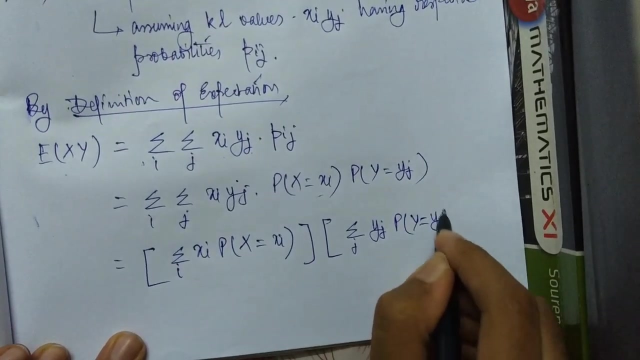 y j. now, if we separate the i's, separate the x and y's term, we have x i into p, x equals x i. this gets separated and y j part j, y j. p y equals to y j. these two get separated and this, as we know, is the 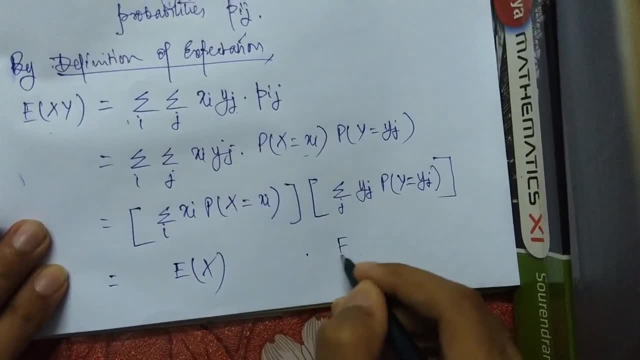 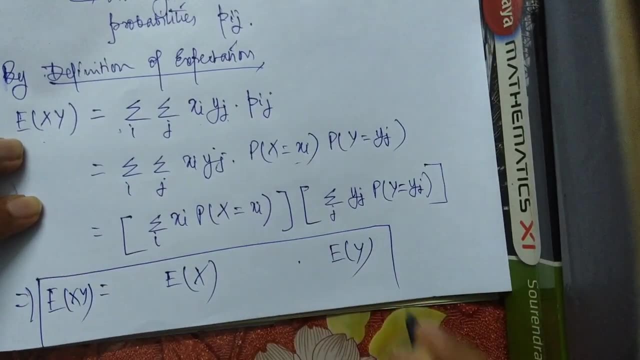 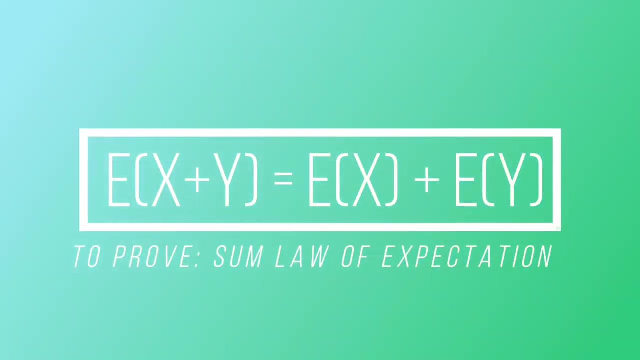 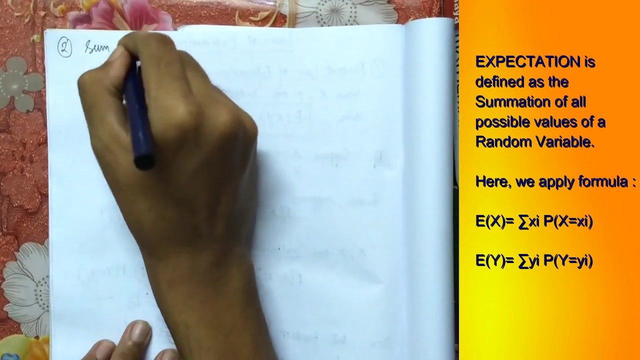 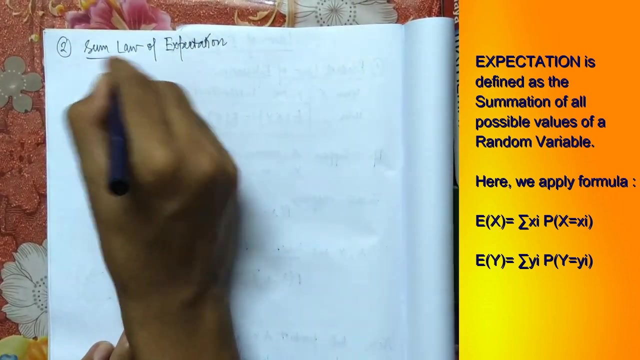 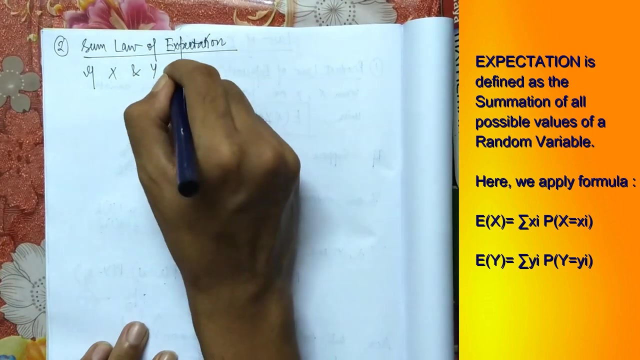 formula of expectation of x, and this is the formula formula of expectation of y, and so we have established that expectation of x, y equals expectation of x into expectation of y. so the next one which we have is known as the sum law of expectation. sum law of expectation has the following statement which says: if x and y are jointly, 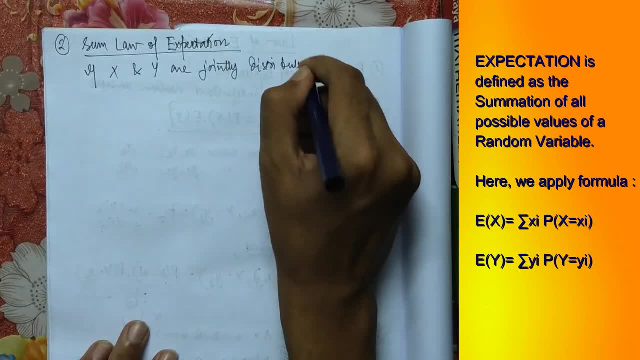 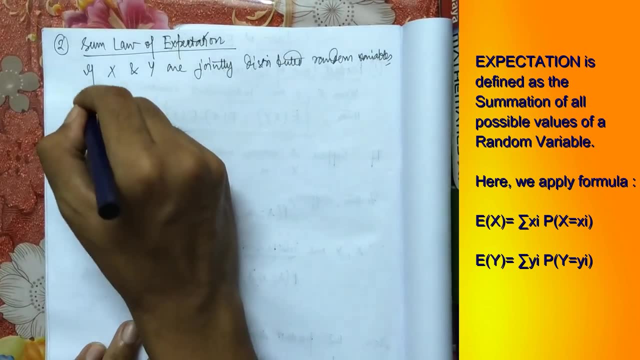 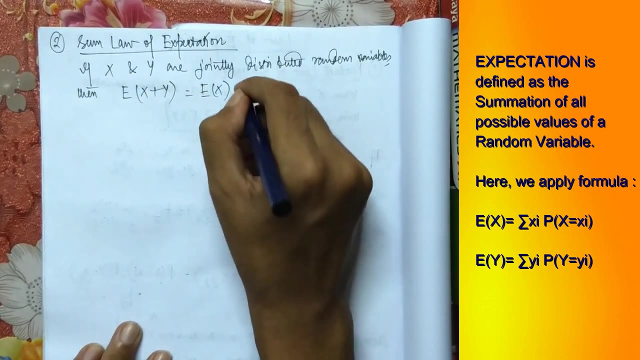 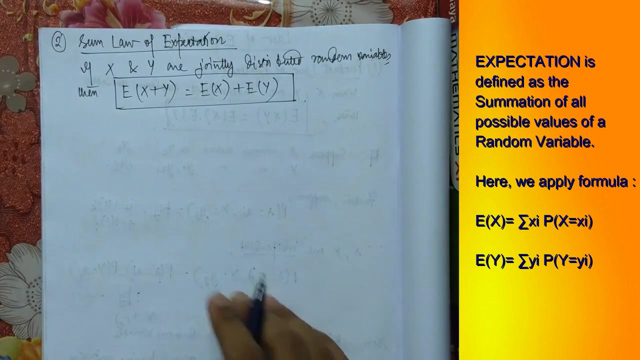 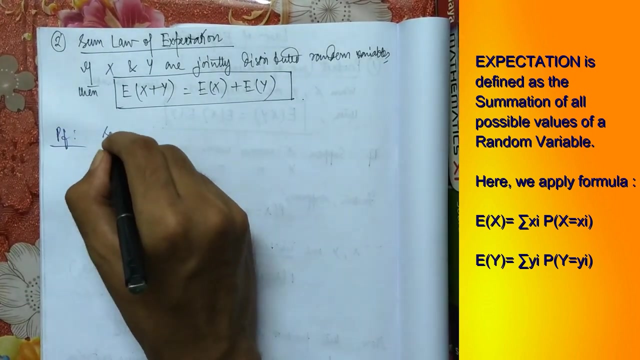 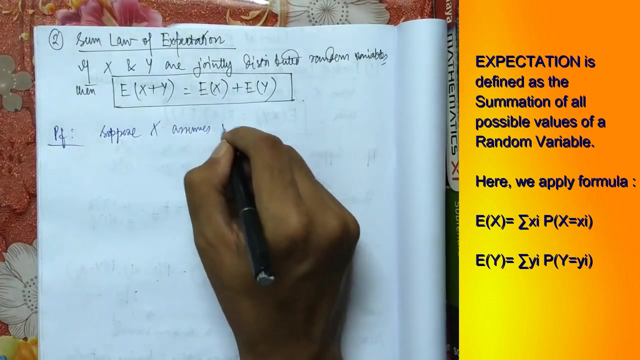 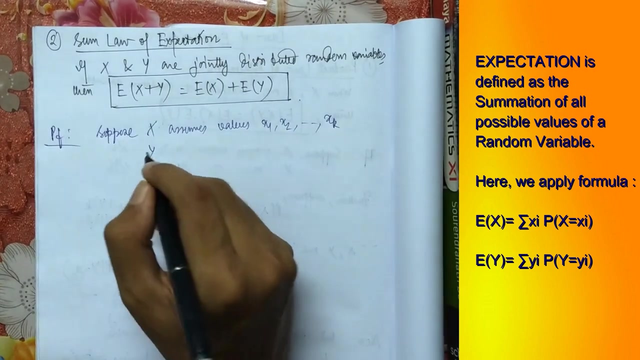 distributed random variables, then expectation of x plus y equals expectation of x plus expectation of y. so here it's obvious that we have to prove this expression. okay, so let us start with it. prove x is a random variable. so suppose x assumes values x1, x2, like this up to xk. this will be same as in the previous product law of. 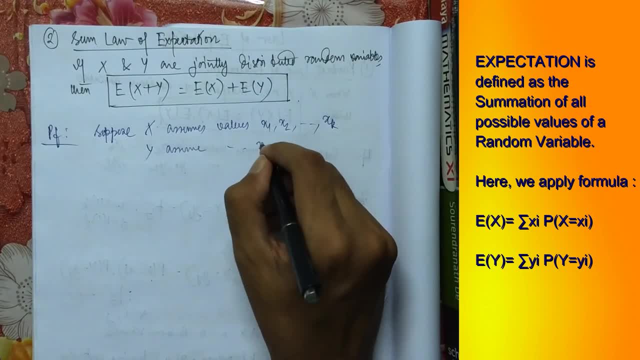 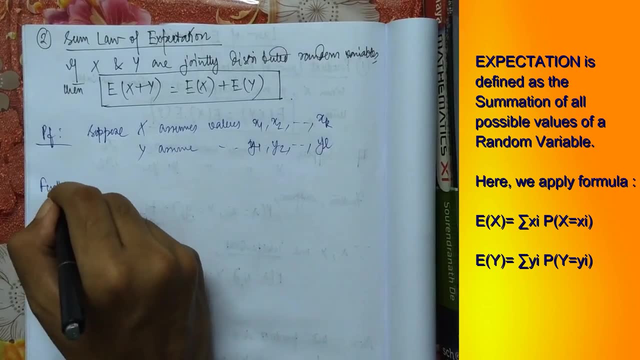 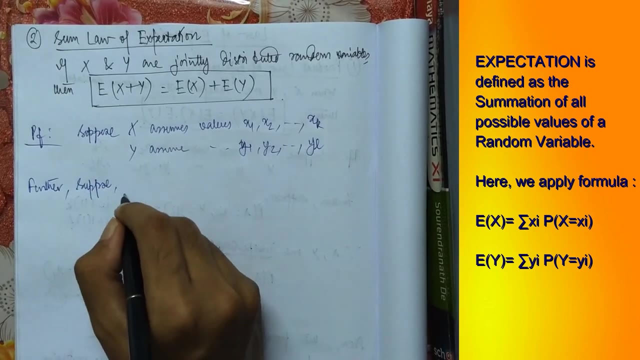 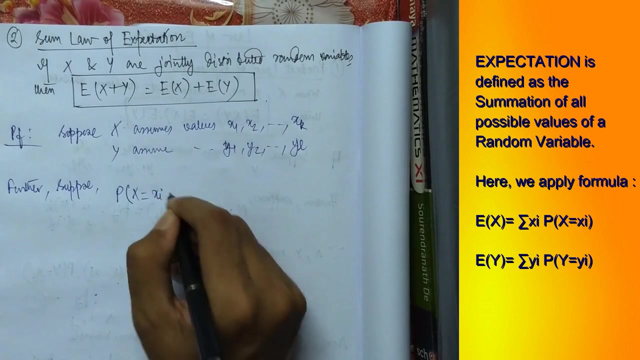 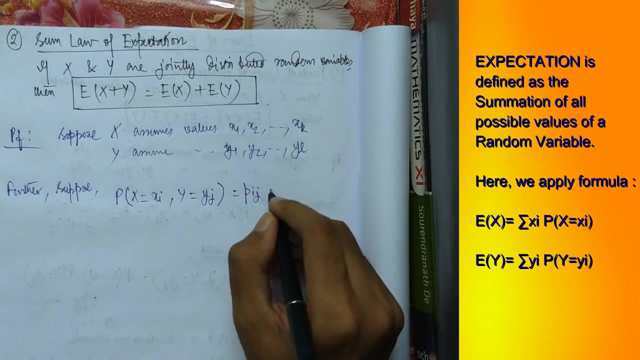 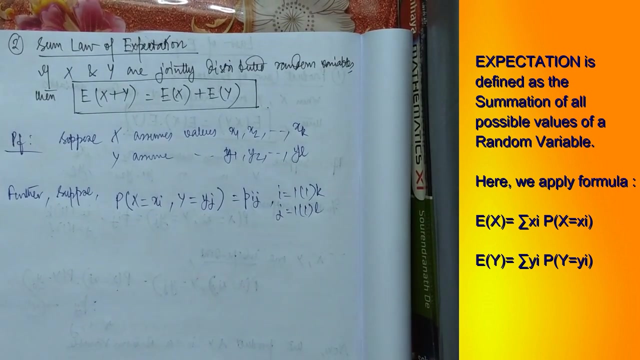 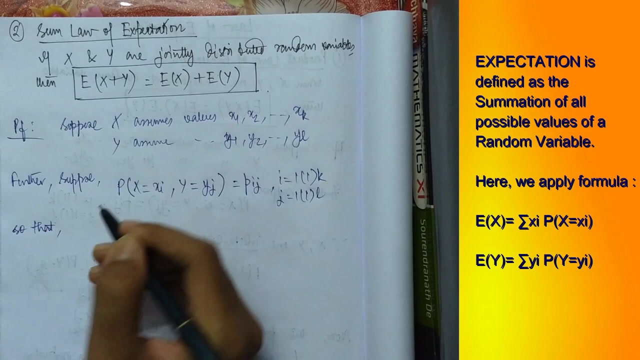 expectation: y assumes values y1, y2, like this yl. further, suppose p, x equals x, i comma, y equals y, j equals pij, where i runs from 1 to k, j runs from 1 to l, so that here on the difference comes that p we denote as p. 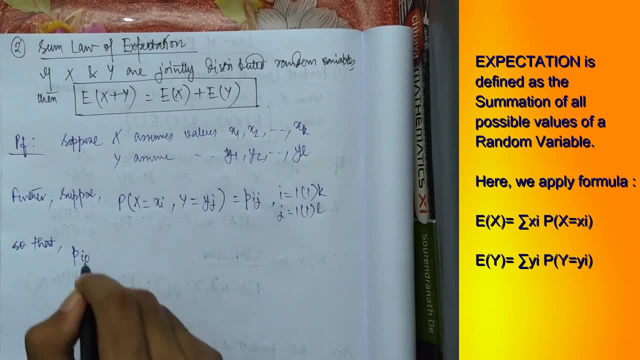 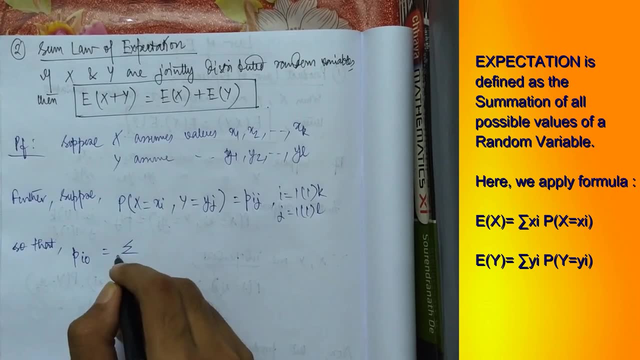 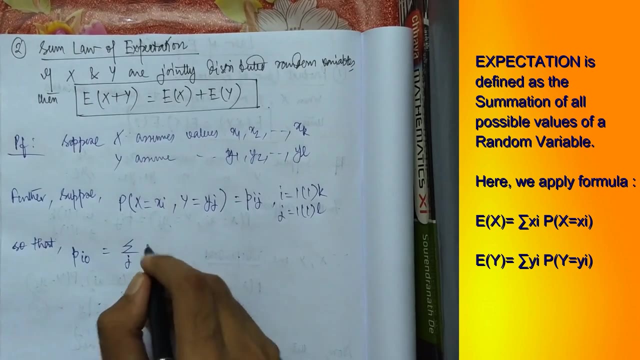 here on the difference comes that p we denote as tr. we put here notation p i 0, as if that i is fixed and j is making the summation. so p i 0 equals summation j, since i 0. so in place of 0 we put in here j, summation j: p i j. 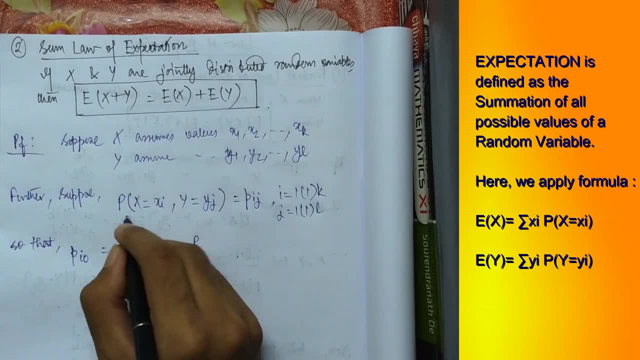 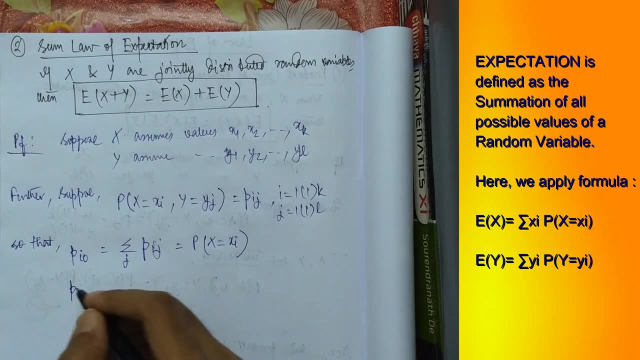 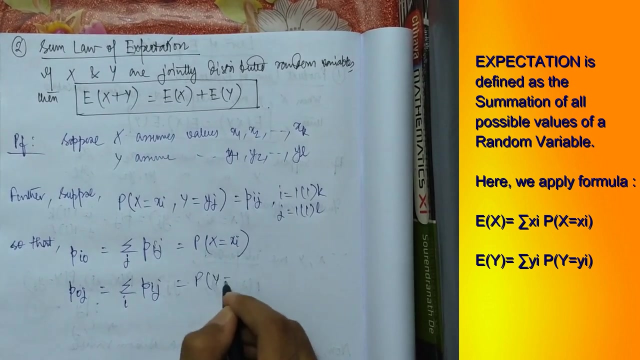 which equals this part. p x equals x- i. similarly, for p 0, j. here what we will put, since we have put in place of i 0, that this will be summation i, p, i, j, which equals the later part. p y equals to y j. now. 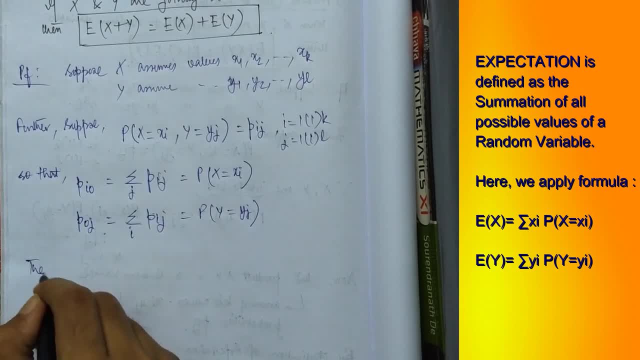 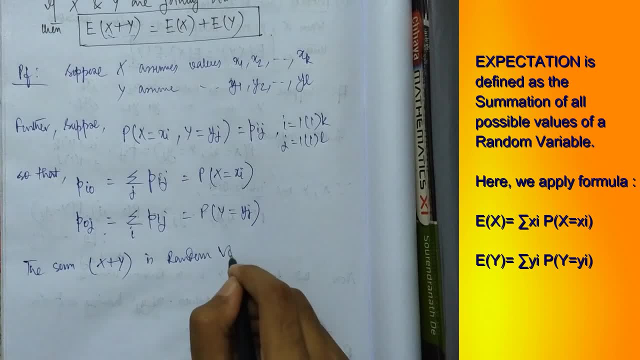 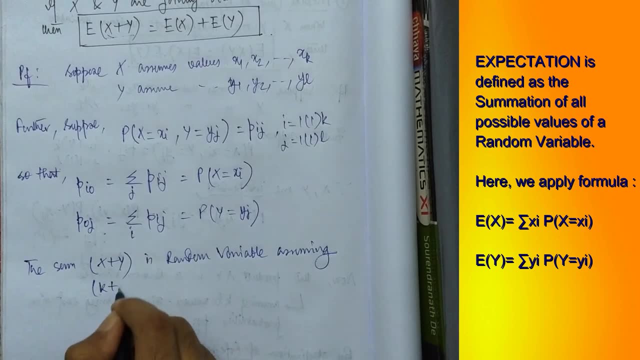 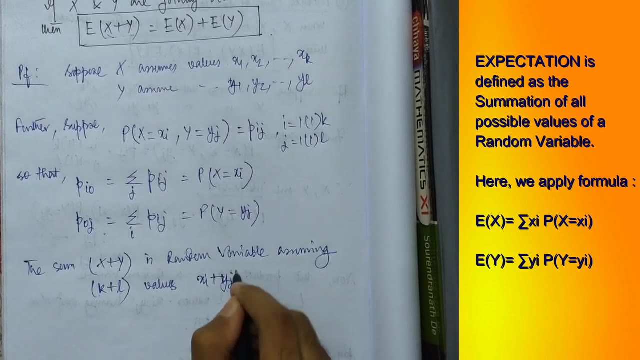 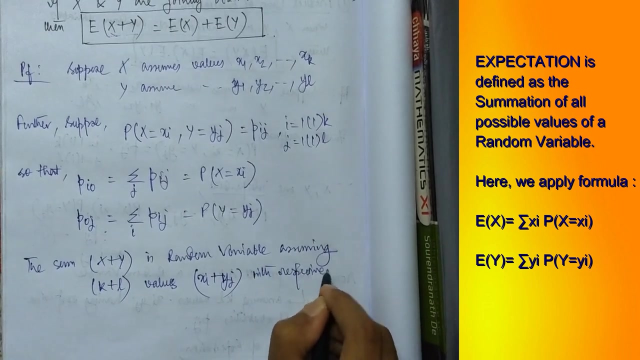 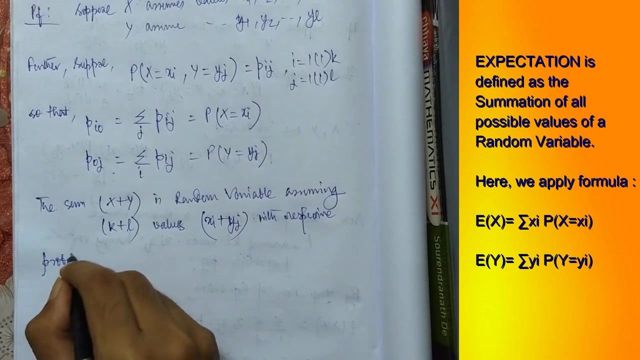 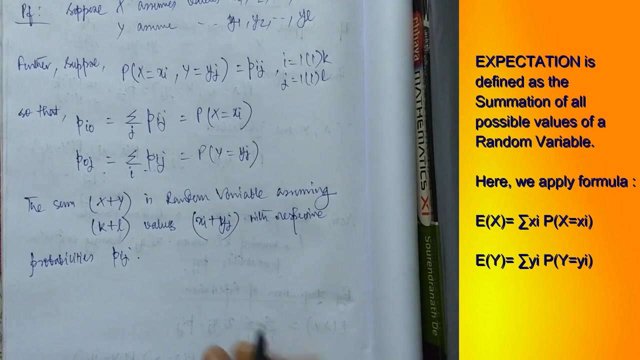 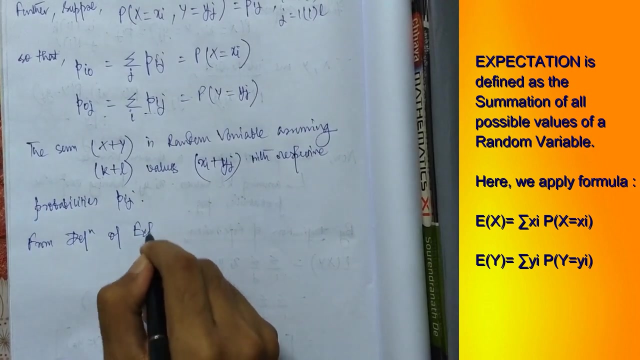 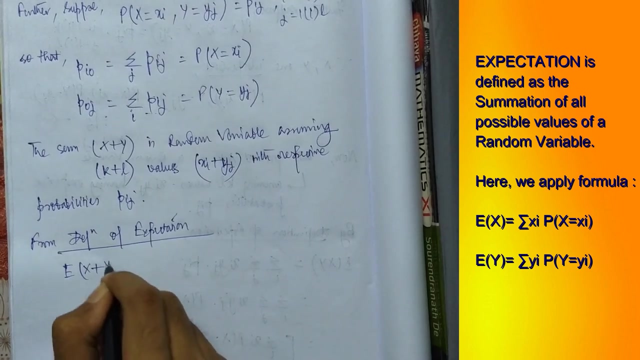 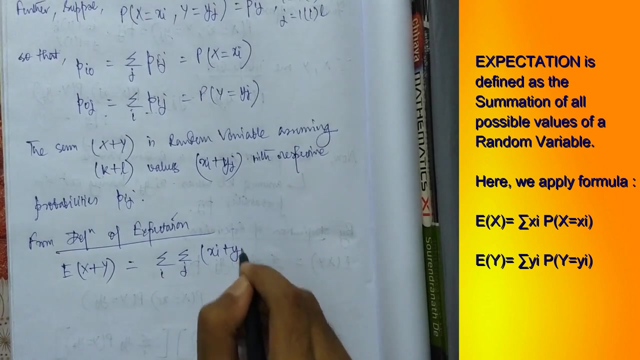 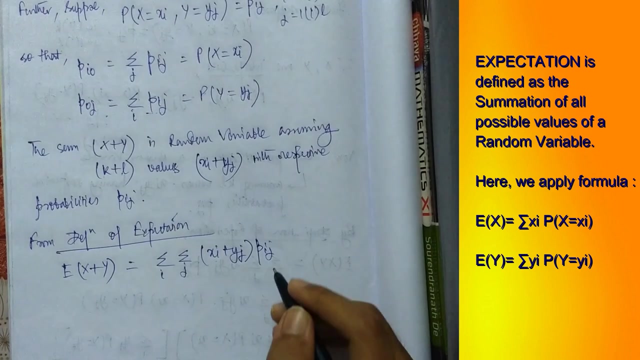 variable, random variable, assuming k plus l values which are x, i plus y, j, with respective probability value which is pij. hence, from the definition of expectation, from the definition of expectation we have in here, that expectation of x plus y equals summation i into summation j, x, i plus y, j into pij. fine, now we will separate this. 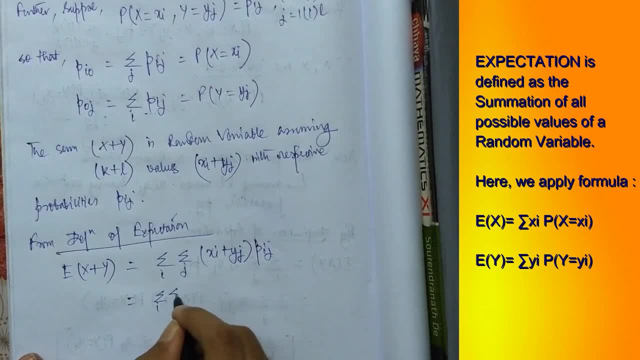 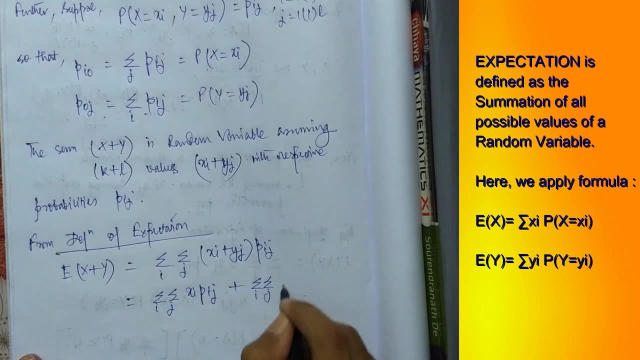 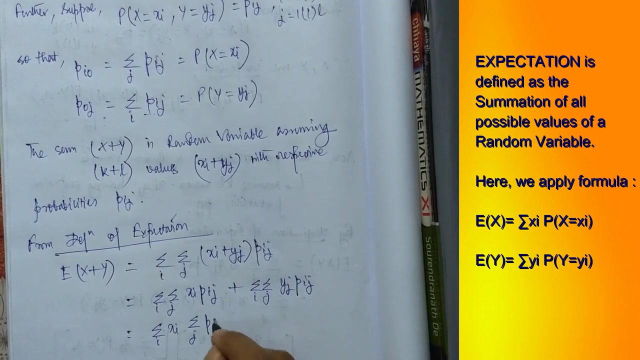 like in the earlier part, summation i, summation j, x, i pij plus summation i, summation j, y, j, pij. now we would separate these two in i's and j's part, summation i, x, i into summation j, pij, plus summation j, y, j to summation i. 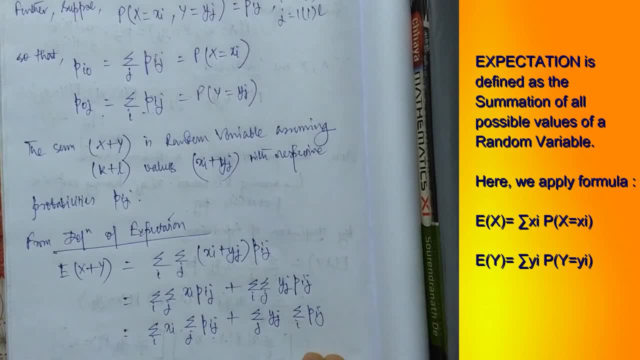 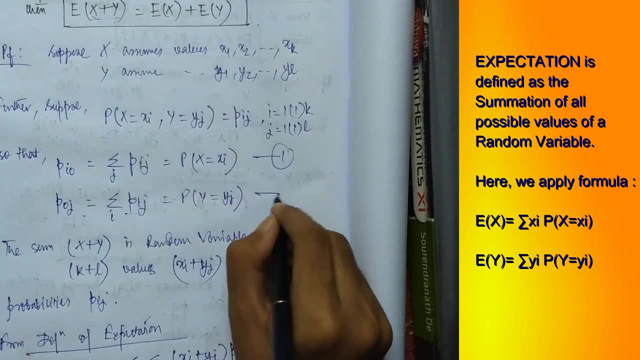 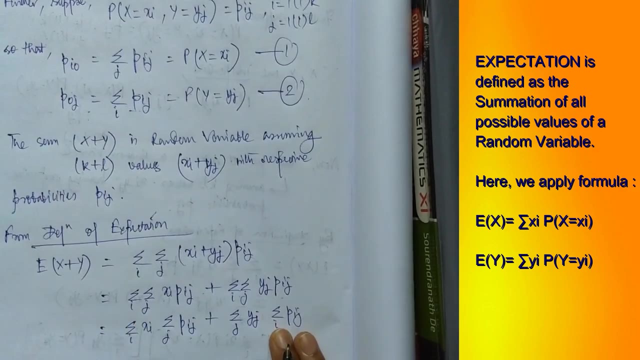 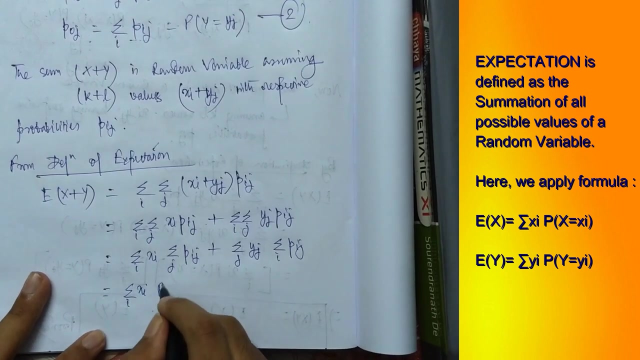 pij. now, earlier we have already taken the relation that summation j pij equals to p x equals to x i and summation i pij equals to p y equals to y j. hence we will put these two relations in here. hence, in this part, summation i x i. summation j pij equals from 1 p x. 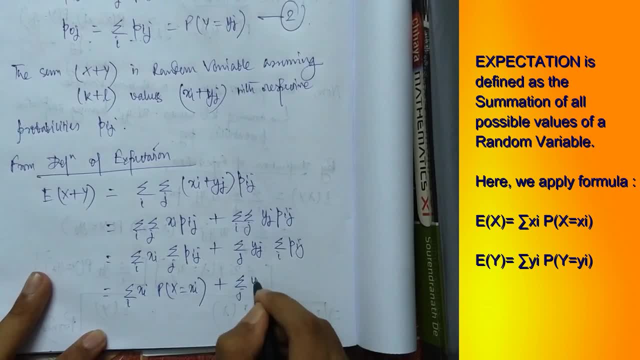 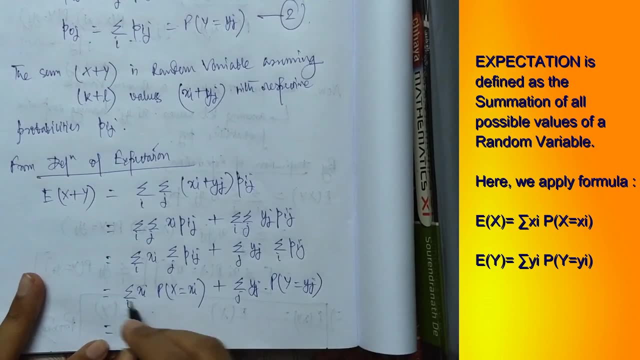 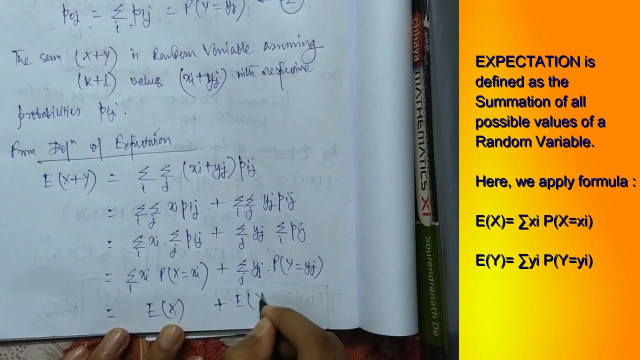 equals x- i and summation j, y, j, pij equals to 1. p x equals x- i and summation j- y, j equals. this becomes p- y equals to y- j. again we have from the definition of expectation: this is known as the expectation of x and this is known as the expectation of y. hence we have expectation. 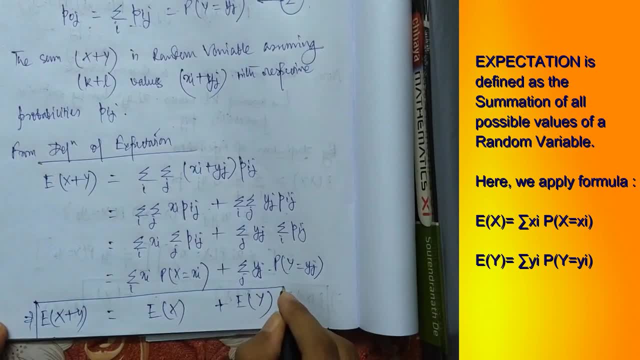 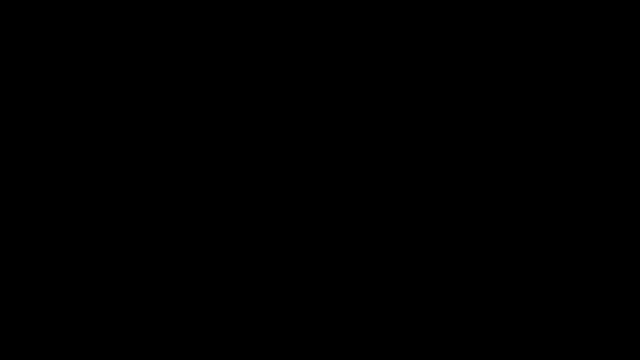